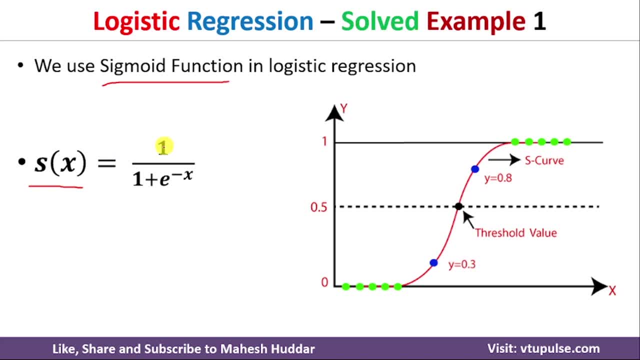 function looks something like this: s of x is equal to one divided by one plus e raise to minus x. in this case, We will get this particular curve Based on the probability. we will decide whether the student will pass or he will fail that particular examination, because we will get the probability. 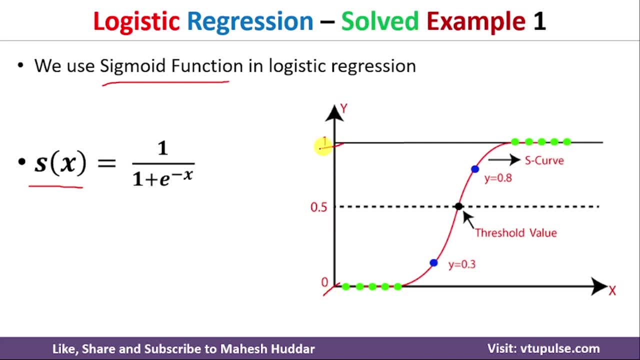 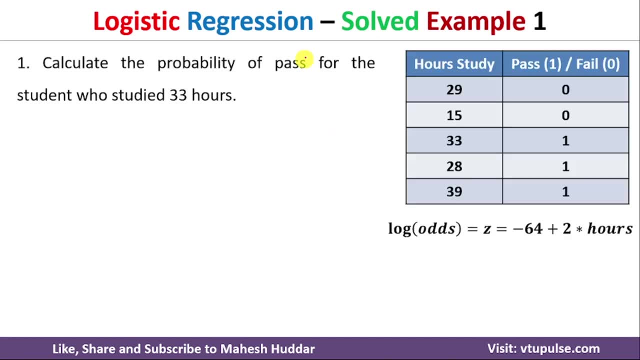 in the range of zero to one. If it is more than 0.5, we will consider that the student will pass. If it is less than 0.5, we consider that the student will fail that particular examination. Now we will continue with the first question, that is, calculate the probability. 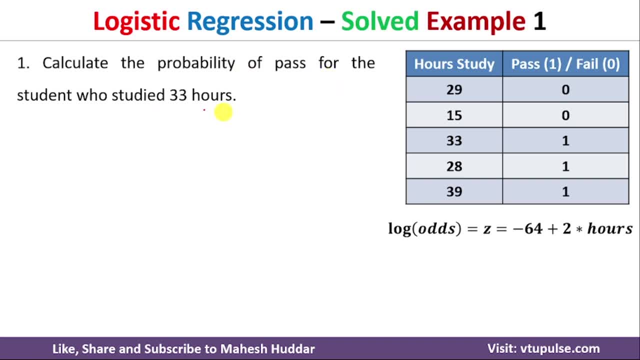 of pass for the student who studied 33 hours. So in this case the number of hours is given to us that is equal to 33.. And we know that the sigmad function s of x is equal to one divided by one plus e. raise to minus x that: 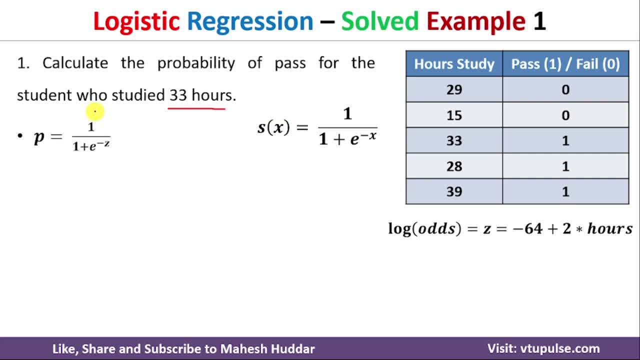 can be written in the form of probability something like this: p is equal to one divided by one plus e raise to minus z. Now we know the equation for z here: z is equal to minus 64 plus 2 multiplied by hours. So if you replace this hours by 33, it looks something. 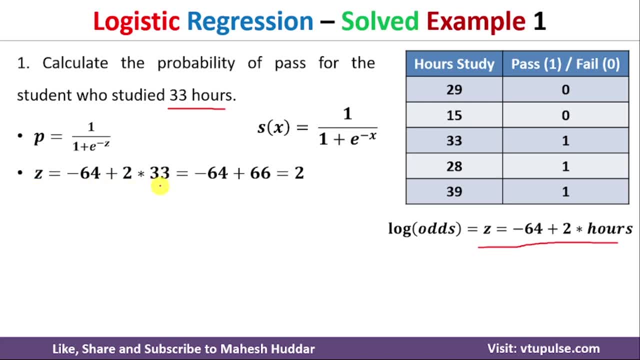 like this: z is equal to minus 64 plus 2 multiplied by 33.. If you solve this equation, you will get 2 as the answer. So the value of z is equal to 2 in this case. Now, if you replace this: 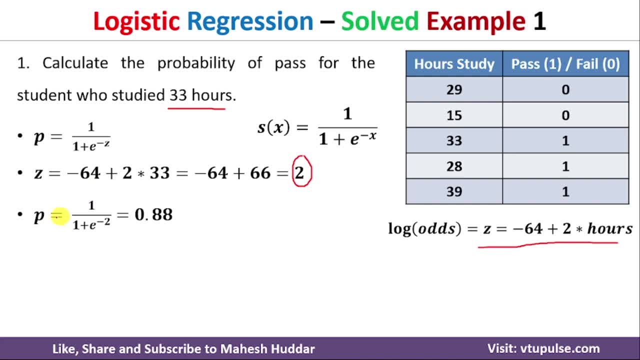 particular z, with the 2, in this particular equation probability is equal to one divided by one. plus e raise to minus 2.. And if you solve this particular equation, you will get 0.88 here. So the probability is equal to 0.88.. The meaning of this particular thing. 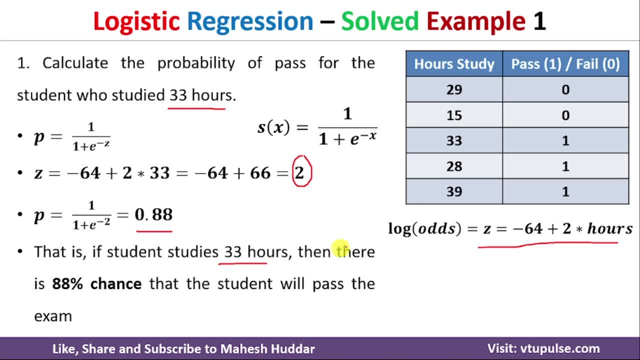 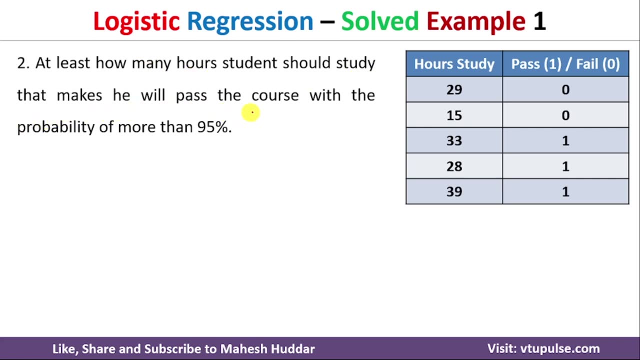 is, if students studies 33 hours, Then there is 88% chance that the student will pass the examination. So this is the answer for the first question. Coming back to the second question- at least how many hours students should study, that makes he will pass the course with a probability of. 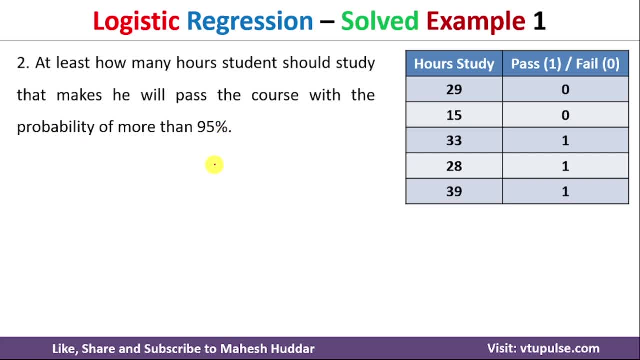 more than 95%. So we need to calculate the number of hours in this particular case. So again, we know the equation for the probability. that is, probability is equal to one divided by one plus e. raise to minus z, which is equal to 0.8.. Now, if you look at the probability, that is equal to 1. divided by 1 plus e, raise to minus z, which is equal to 0.8.. So if students studies 33 hours, then there is 88% chance that the student will pass the examination. So 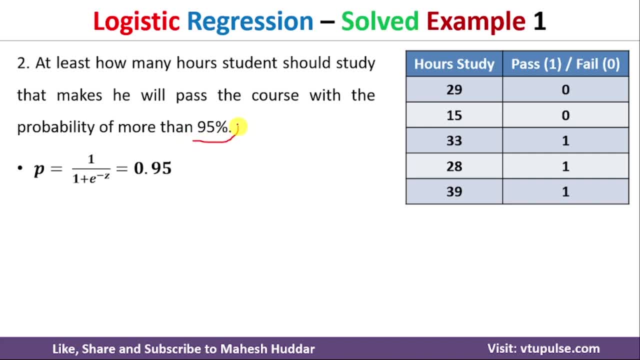 0.95 here, because probability is given to us that is 95 percent. that means 0.95 in this case. now what we do is we will try to simplify this equation. i will take 1 plus e raised to minus z on this side it will become 0.95 multiplied by 1 plus e raised to minus z is equal to 1 here. 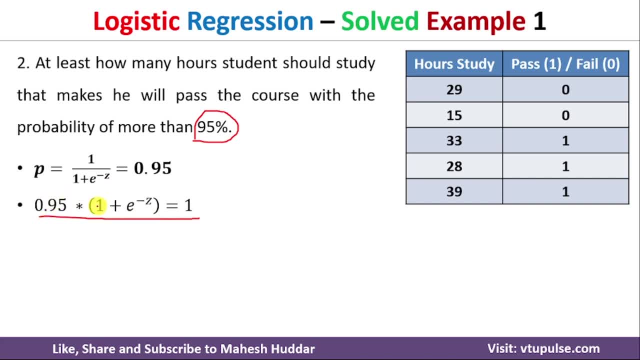 so that is what i have written here. i will take this minus 0.95 inside, so it will become 0.95 plus 0.95 multiplied by e raised to minus z, which is equal to 1, and if you simplify that thing it will. 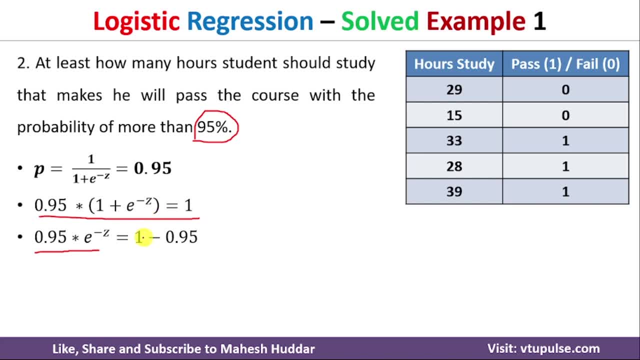 become 0.95 into e raised to minus z, plus equal to 1 minus this particular 0.95 will come on this side. now, uh, i will get this particular equation something like this: e raised to minus z is equal unto. this is equivalent to 0.05 divided by 0.95, and if you solve it, you will get 0.05 to 6 here. 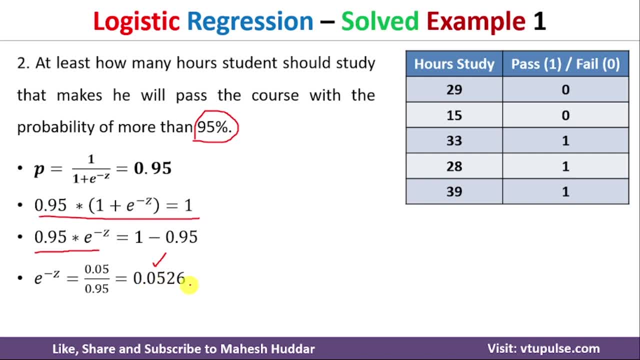 so e raised to minus z is equal unto 0.0526. we need the value of z. so once you know the value of z, then you can calculate the number of powers. so what we do here is we will take a natural logarithm on both the sides. so ln of e. 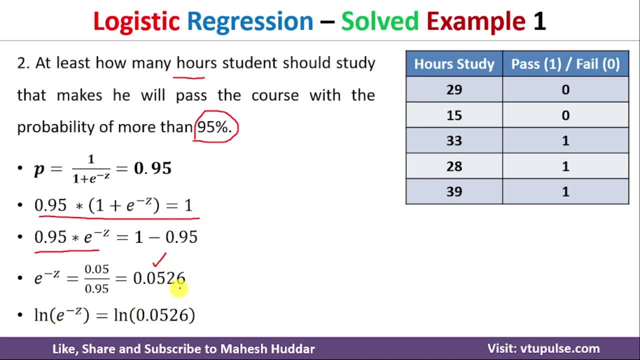 raised to minus z is equal unto ln of 0.0526. now we know one property of a natural logarithm, that is, ln of e raised to x is equivalent to x here. so ln of e raised to anything is equivalent to same over here. so in this case we have ln of e raised to minus z. the meaning: 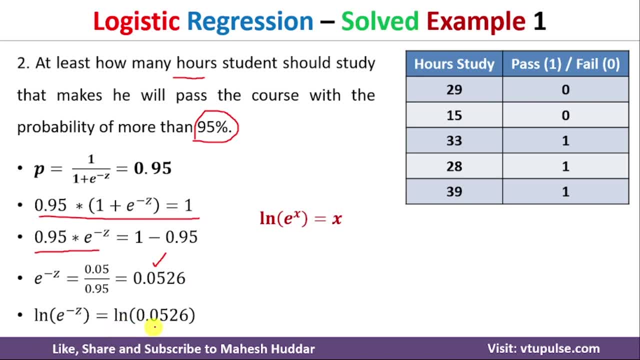 of this one is on the left hand side. we will get minus z right hand side. it is ln of 0.0526 here. so that is what i have written here, and if you simplify this ln of 0.0526, we will get minus. 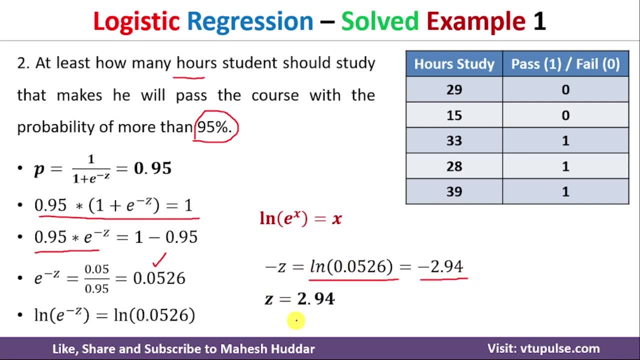 2.94. that means the value of z is equivalent to 2.94 here. so we have calculated the value of z in this case, which is equivalent to 2.94. once you calculate the value of z, that is, z is equivalent to 2.94- we know the integral of z is equal to 1.9. and if you calculate the value of x, that is equal to 2.94. we know the. 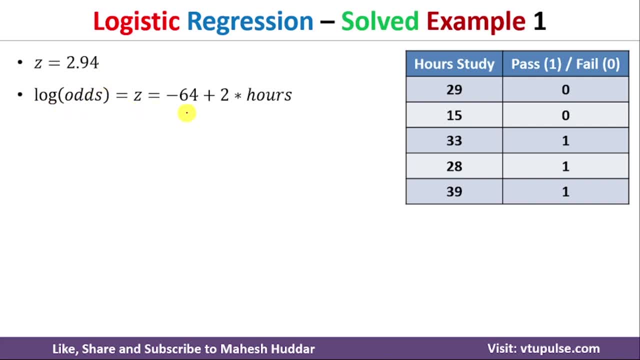 equation for log of odds that is equivalent to z, which is equivalent to minus 64 plus 2 times hours here. so in this case we will replace this particular z by 2.94. it will become 2.94, which is equivalent to minus 64 plus 2 times hours. here i will take this particular 64 on the other side. 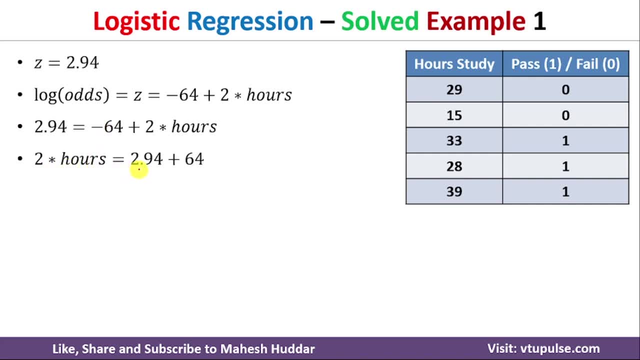 it will become: 2 multiplied by hours is equivalent to 2.94 plus 64. 2 multiplied by hours is equivalent to: if i add these two things, it will be 66.94 here. now i will take this particular 2 on the other side. so hours is equivalent to 66.94 divided by 2, which is equivalent to 33.47 hours here. 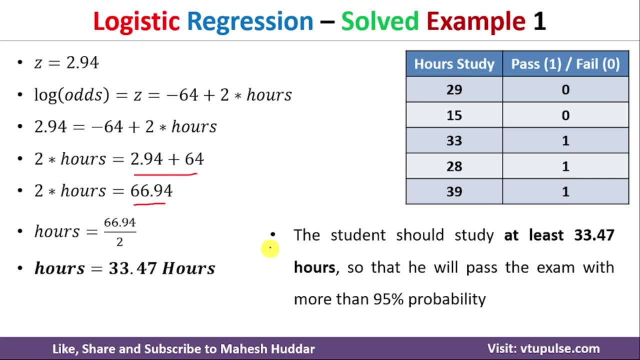 the meaning of this particular thing is: if the student has studied at least 33.47 hours, then he will pass the exam with more than 95 percent of probability here. so he has to study at least 33.94 hours so that he will pass the examination with more than 95 percent probability in this case. 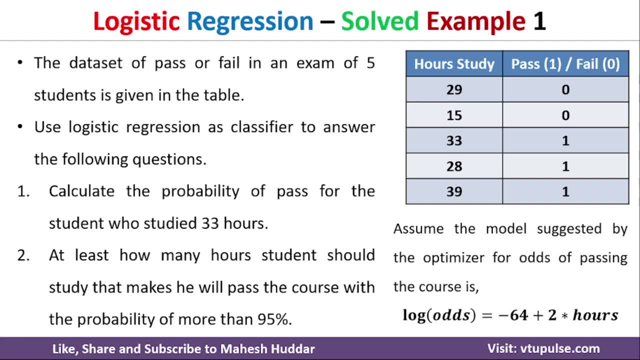 in the previous videos i have discussed what is logistic regression, how logistic regression works and what are the advantages and disadvantages of logistic regression algorithm. the link for that video is given in the description below. do watch that particular video to understand the basic concept of logistic regression. in this video i have discussed given 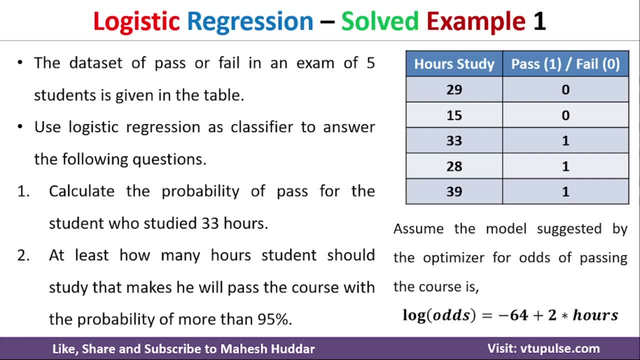 the logistic regression classifier by the optimizer, how can we calculate the probability of a particular class with the value of independent variable? in this case, the independent variable is hours here. so if 33 hours is given, how can we calculate the probability? and if the probability is given to us, how can we calculate the value of independent variable? that is, 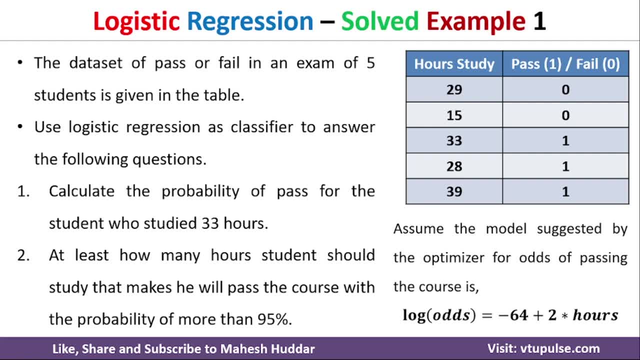 hours here. i hope the concept is clear. if you like the video, do like and share with your friends. press the subscribe button for more videos. press the bell icon for regular updates. thank you for watching.